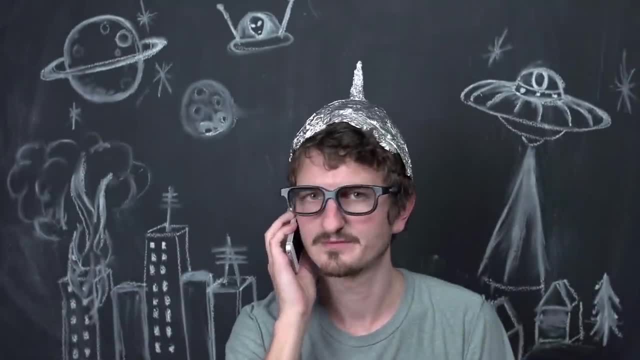 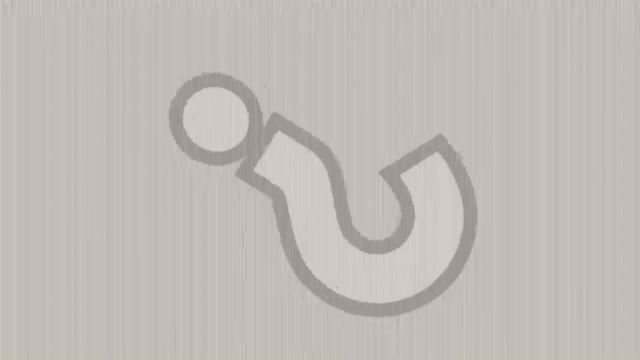 geometry or whatever else—in order to prove something, you have to rely on proofs that already exist. Those proofs rely on other proofs, which rely on other proofs down and down the line, until you get to the basic assumptions that you can't really prove—they just feel right. 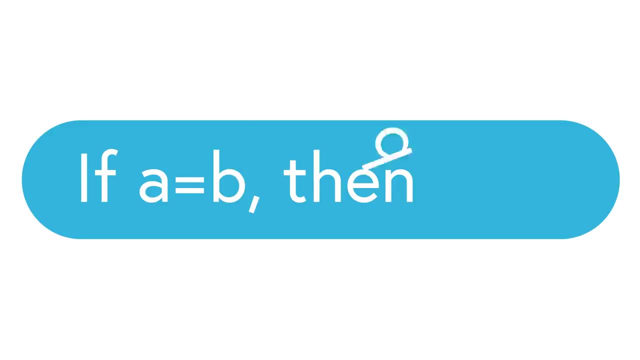 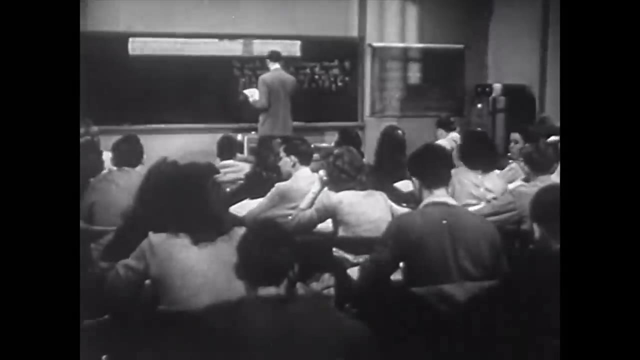 Like. one of these assumptions for algebra is that if A equals B, B also equals A. If I asked you to prove that to me, you would probably laugh politely and then stop talking to me for forever. But up until the 20th century, these basic assumptions were different for each. 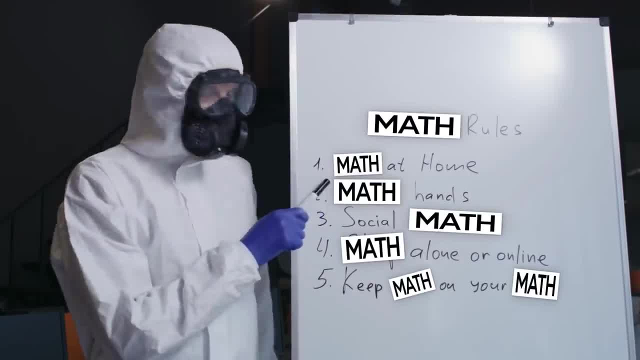 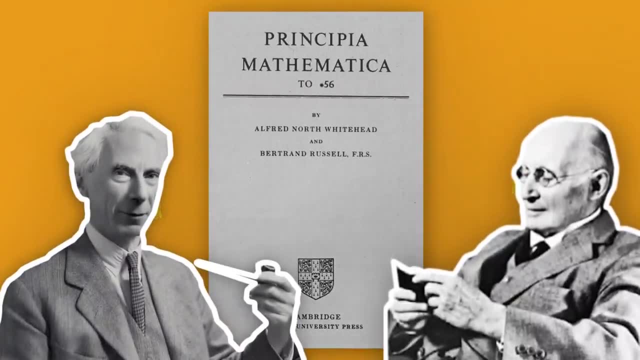 different branch of mathematics—there wasn't one set of rules that you could use to prove everything that's true in math. Principia Mathematica was an attempt to fix this. Its authors wanted to derive a complete system of mathematics from pure logic, starting with 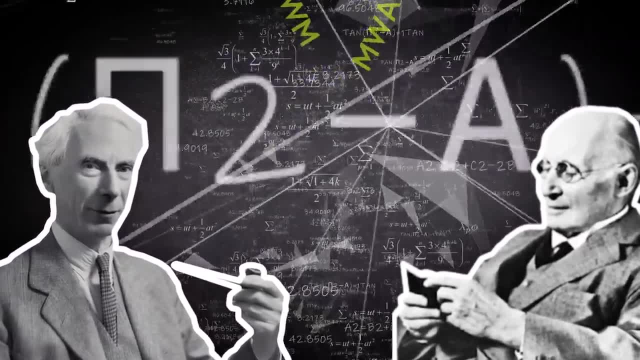 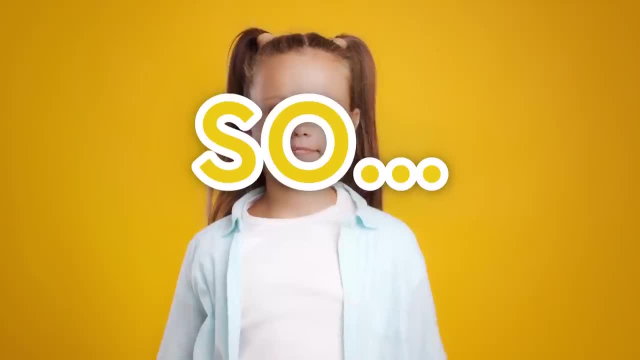 just a few key assumptions and taking small logical steps from there to build out everything we know about math. Just to be clear, this didn't actually work—turns out it's actually impossible to do that without any holes. So this whole book is kind of useless. But it did result in a 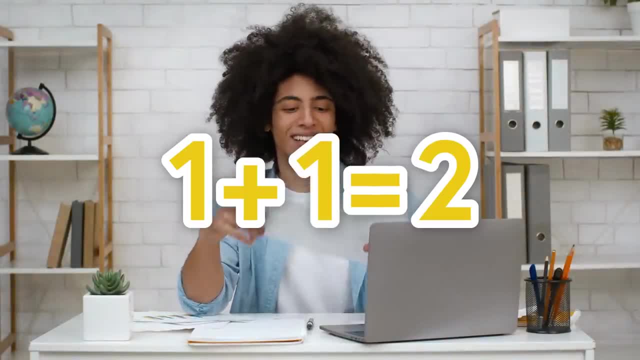 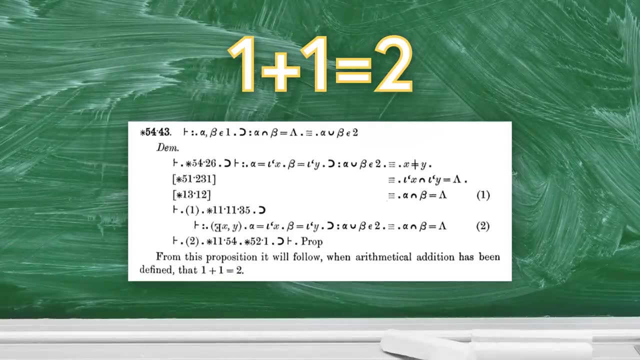 very weird and very convoluted proof that 1 plus 1 equals 2 along the way, and I thought that was kind of funny. so here we are. This is the section that proves 1 plus 1 equals 2—or at least this. 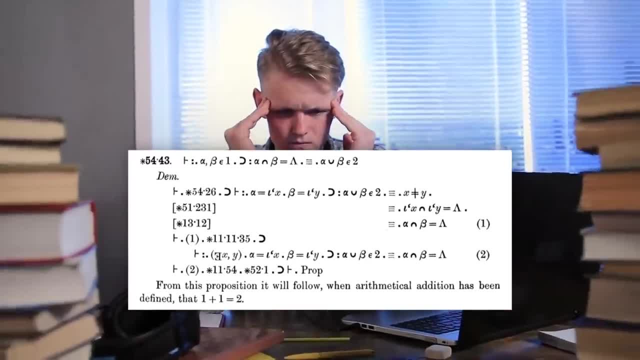 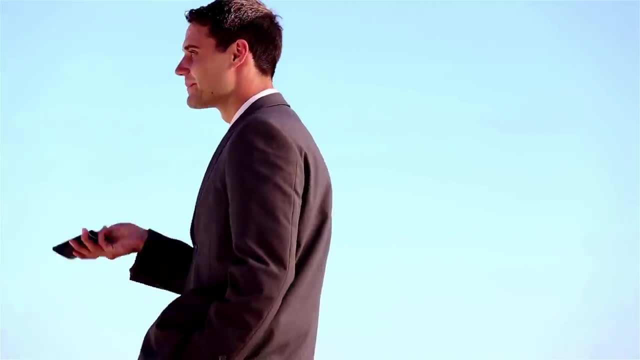 is the main chunk of the proof. If you're a normal person with a normal brain, you're probably looking at this and thinking, ow oof, my normal brain hurts. But if you have a PhD in mathematics, then you'd probably be doing something more important than watching this video. 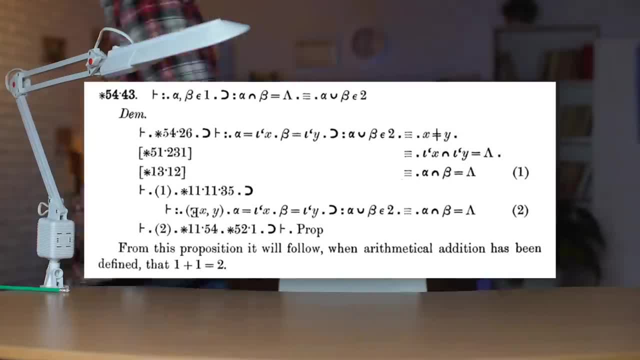 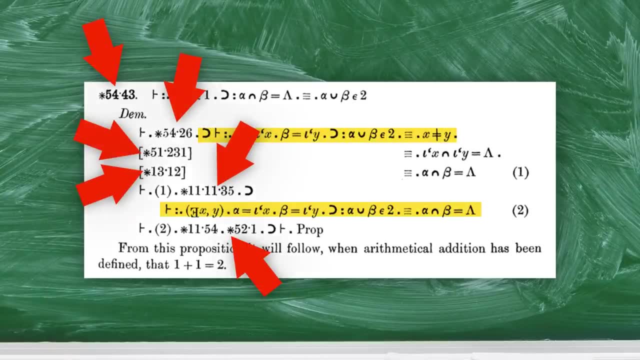 If you did, though, you'd still probably have a really hard time figuring out what any of this means, And that's because a lot of these symbols are super old and aren't used anymore, and almost all of these numbers are just references to earlier sections of the book, which has been 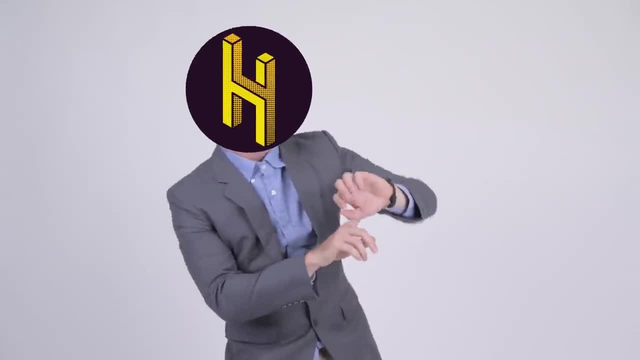 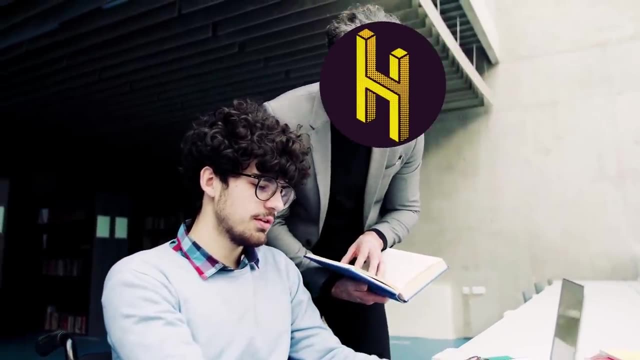 read in its entirety by almost nobody. This shows up on page 360, and it's built on a lot of other proofs and definitions that I don't really have time to explain, so let's go ahead and walk through each line together, and we'll all come out of this somehow more annoyed than when we began. 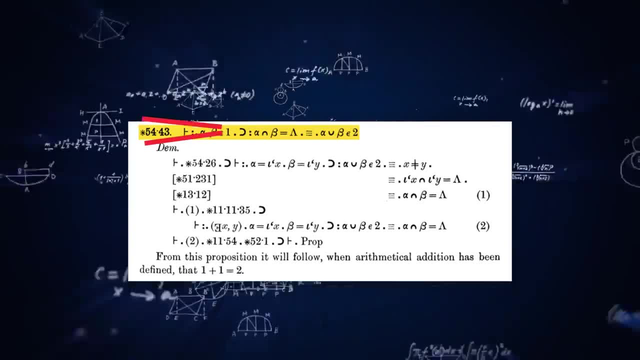 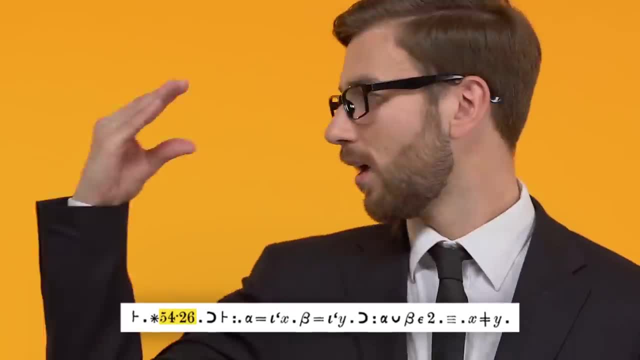 The first line basically lays out what the whole section is trying to prove, so we don't have to worry about that for now. The proof begins here, which is mostly built off an earlier section of this book, 54-26.. I'm just going to tell you what it means, because if I had to explain how 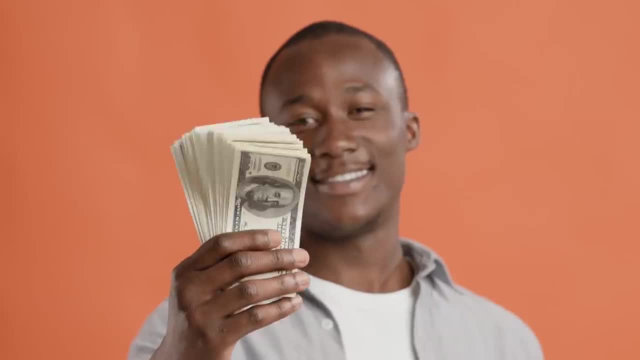 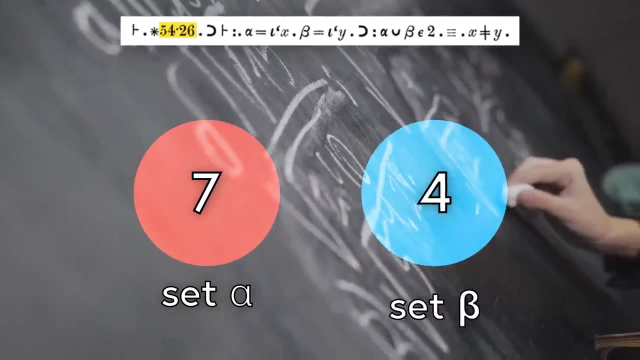 they proved this was true too, then I'd just end up reciting the whole section. Basically, this theorem states that if A is a set of numbers with exactly one number in it and B is a set of numbers with exactly one number in it, then a set of numbers that contains all the 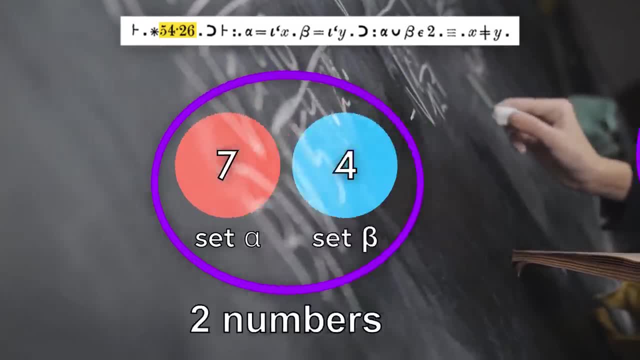 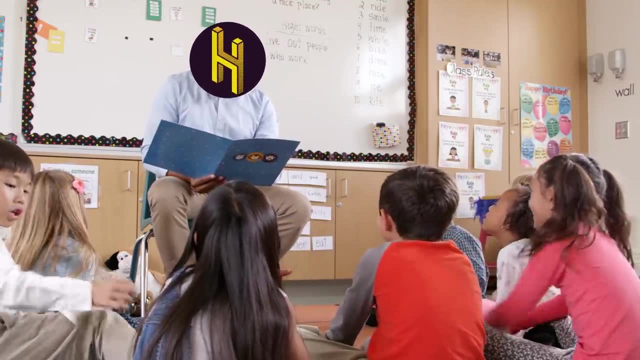 numbers from A and B will only have two total numbers if the numbers contained within A and B aren't equal to one another. Yeah, that seems kind of obvious, but you're watching a video about why one plus one equals two right now, so you're in no place to judge Now. these next two lines are: 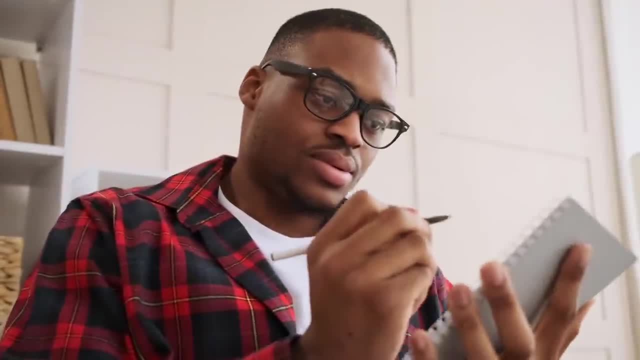 saying something even more obvious—kind of something so obvious that it's hard to even describe what it is that they're trying to prove. They're saying that A is a set of numbers with exactly one number in it, and B is a set of numbers that contains all the numbers from A and B. 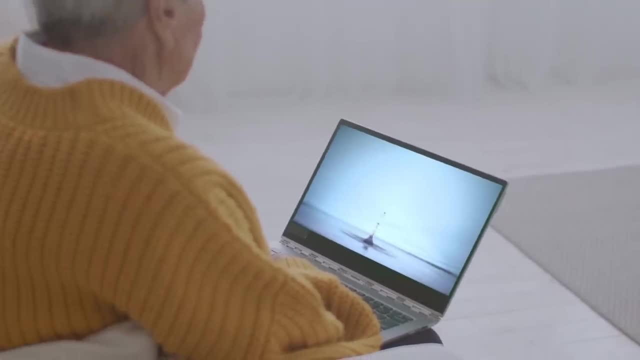 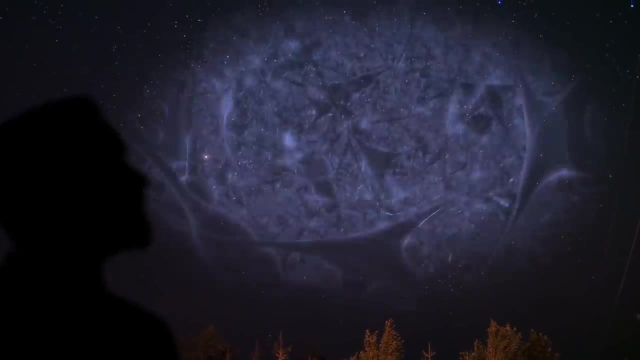 Like: have you ever encountered something so simple that it was impossible to comprehend? Have you ever stared into the ceaseless void of space, not able to see anything at all, but still paradoxically incapable of grasping what it is you're seeing? for it is the very absence of 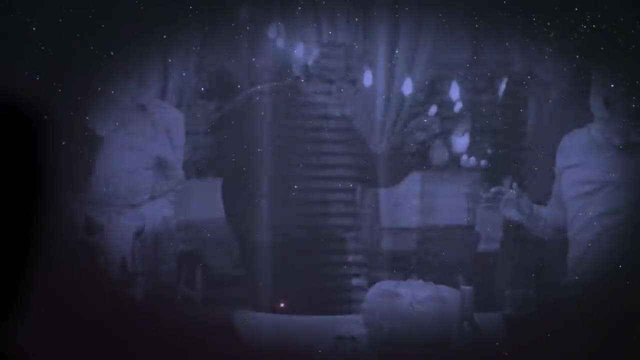 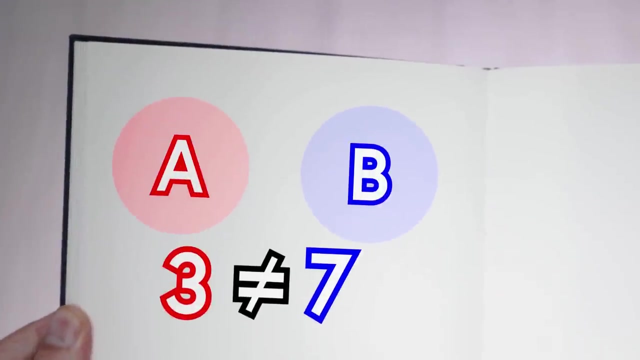 light—the very absence of information itself that the human mind cannot possibly hope to comprehend. These lines are kind of like that. The argument here is that if the numbers contained within sets A and B are different, that is the same thing as saying that the 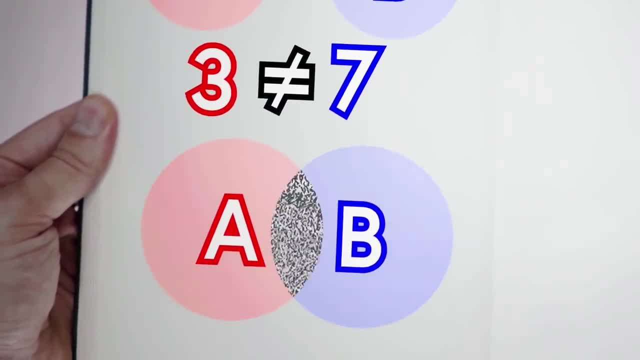 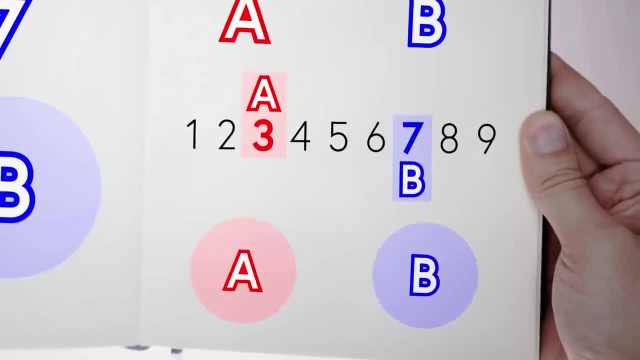 intersection between sets A and B is the set with no numbers in it. Or in other words, if A and B each have one number and those numbers are different, then A and B have no overlap—the sets themselves are also different. Cool, I guess. 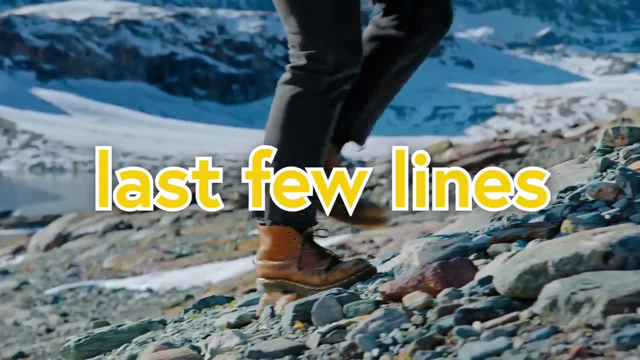 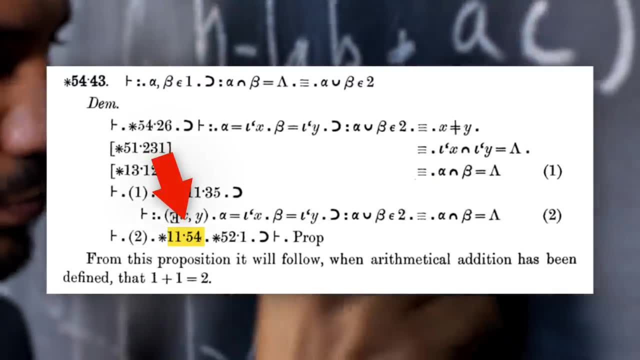 And that leads us to the conclusion with these last few lines. It brings in some other sections to tie everything together, but they're so technical that they're not really worth talking about Like this one. 11-54, literally just means that if two things exist, 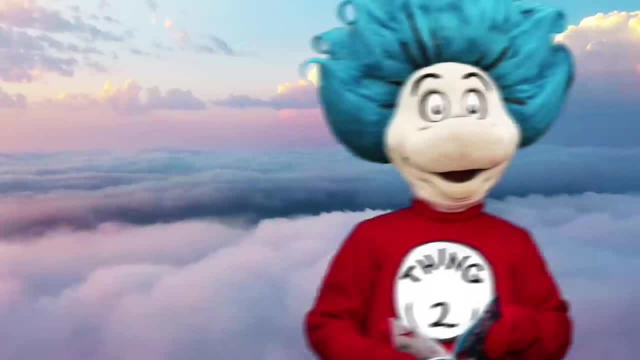 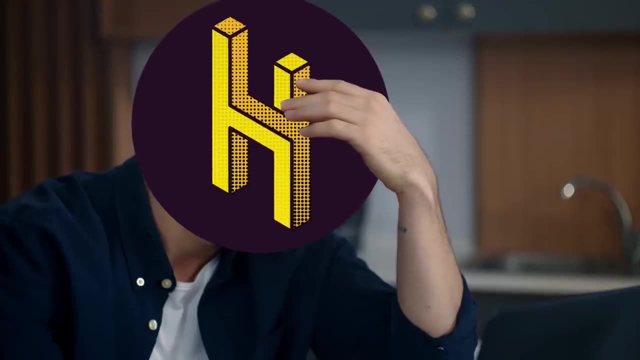 you can conclude from it that one of those things exists and also that the other thing exists. That's not a joke—I'm not joking. There's a whole section of this book dedicated to proving that. I can't believe. I made my writer suffer through. 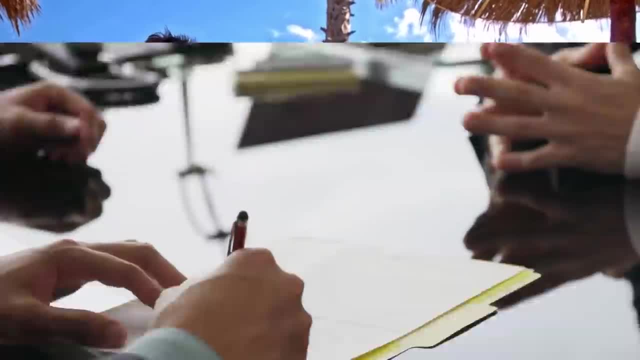 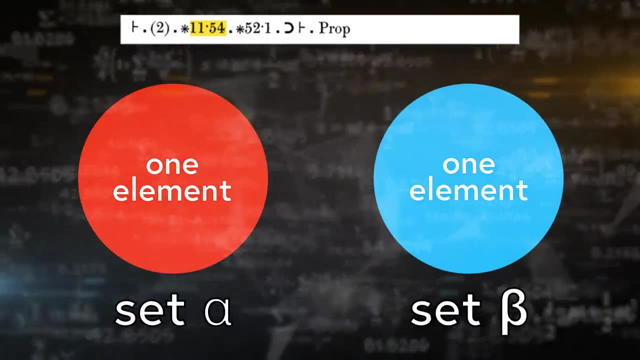 reading this stupid book. I think I'm going to give him a week of paid time off. and this video is a legally binding agreement—oh nice try. Anyway. this conclusion essentially states that if set A and set B each have one element, 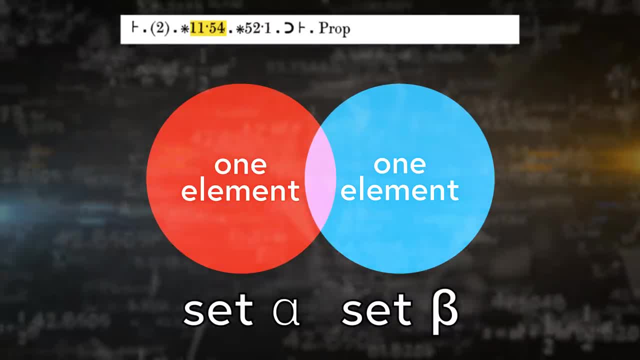 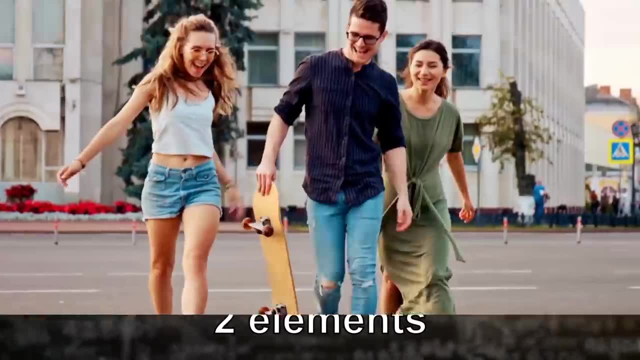 and the intersection of A and B is the set with no elements, then you can prove that a set containing all of the elements of set A and set B has exactly two elements. Or, as the cool teens would put it, if you have a group of one thing and combine it with a group of a different thing. 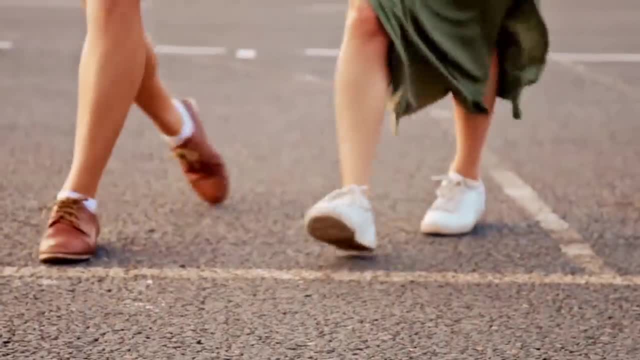 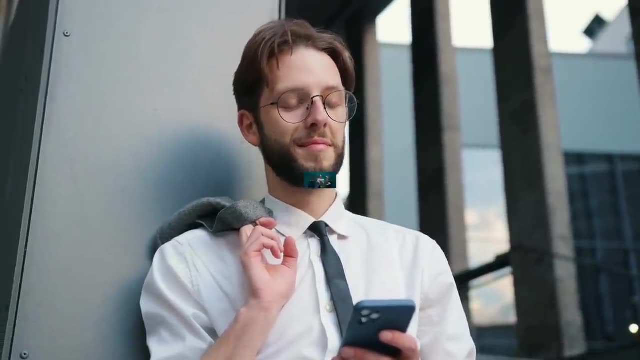 you get a group of two things, So one plus one equals two. Now that you know what one plus one equals, you might think you know everything you need to know about the world, but you're wrong. The world is a complicated and rapidly changing place.